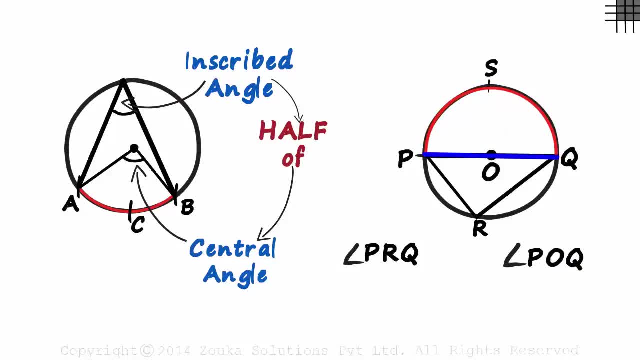 Doesn't quite look like an angle as it is a straight line, But it definitely is. It's this angle. The inscribed angle is half of the central angle. Do we know angle POQ? Of course, If it is a straight angle, it will measure 180 degrees. 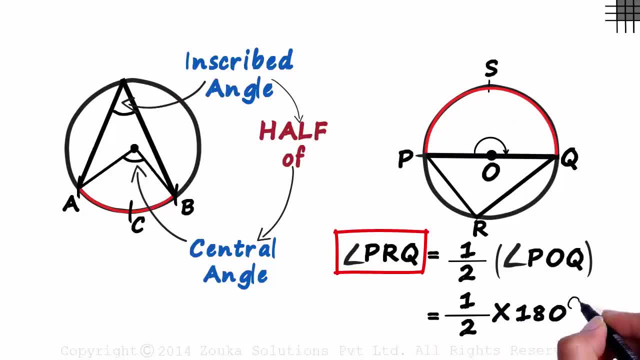 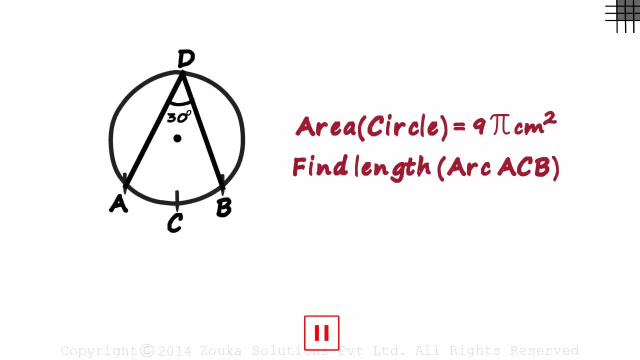 Angle. PRQ will measure half times 180 degrees, which will be 90 degrees. It is a right angle. PQ is the diameter and two semi-circles are formed. Here is a typical kind of problem that you might see in your exams 2.. 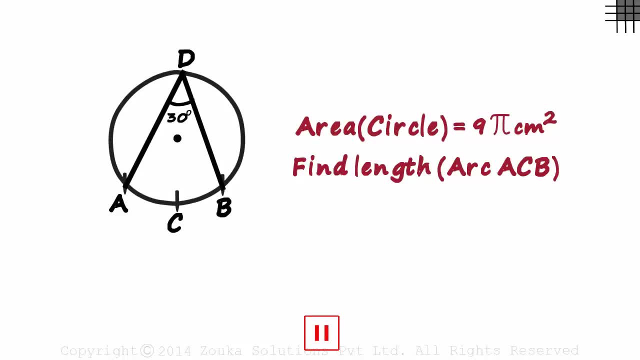 GOT, 2. GOT, 3. GOT, 5. GOT, 6. GOT, 7. GOT 8.. Given the measure of angle, ADB is 30 degrees, The area of the circle is given as 9 pi And we are asked to find the length of arc ACB. 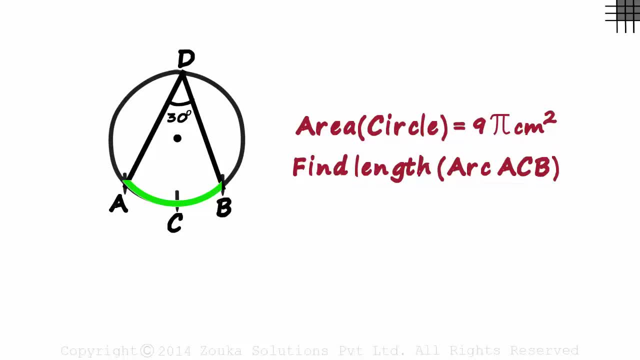 So we have been asked to find this curved length. All we have is the area of the circle and the measure of this angle. What do we need to find the length of an arc? Yes, The first thing required is its central angle. We can draw two radii like this and call its central angle theta. 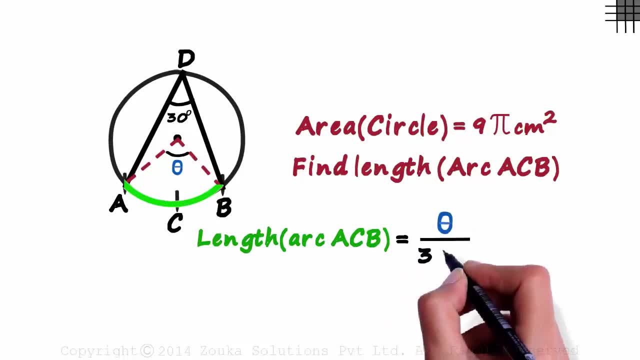 The length of arc ACB will be theta over 360 degrees times the circumference, which is 2 pi r. Out of the two unknowns on the right, we have none, But can we find them? Probably Theta is the central angle of arc ACB, which is the arc subtended by this inscribed angle. And we learnt that the inscribed angle is the central angle of arc ACB. And we learnt that the inscribed angle is the central angle of arc ACB. And we learnt that the inscribed angle is the central angle of arc ACB. 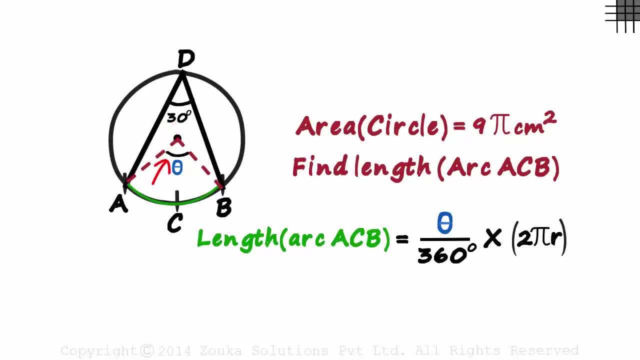 And we learnt that the inscribed angle is exactly half of the central angle. that subtends the same arc. 30 being half of theta implies that theta will be twice that of 30. It will be 2 times 30 degrees, which equals 60 degrees. 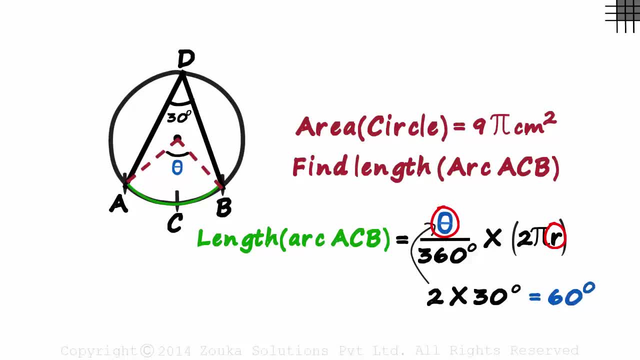 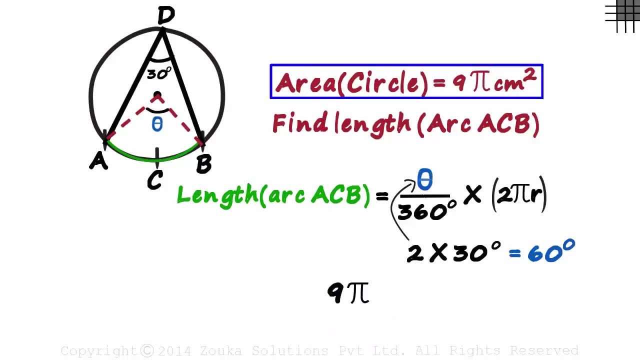 We have found one unknown. How do we find the radius? Don't forget, we have also been given the area. The area is 9 pi And the area of a circle is pi r square. Solving this gives us the value of r as 3 centimetres.